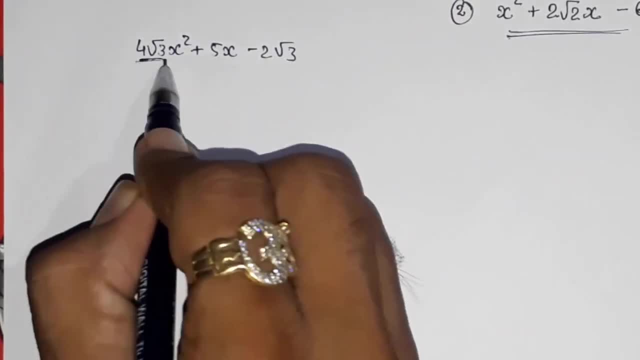 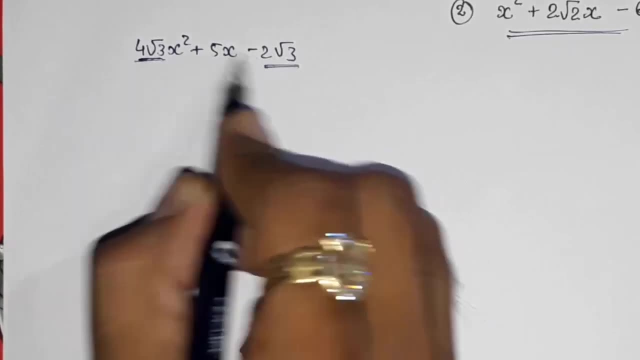 sum that way only. first we have to multiply the coefficient of x square, and the last c means a and c. that will be 4 into 2, 8 minus 8 and 3 into 3. so root. 3 into root, 3, 3 so minus. 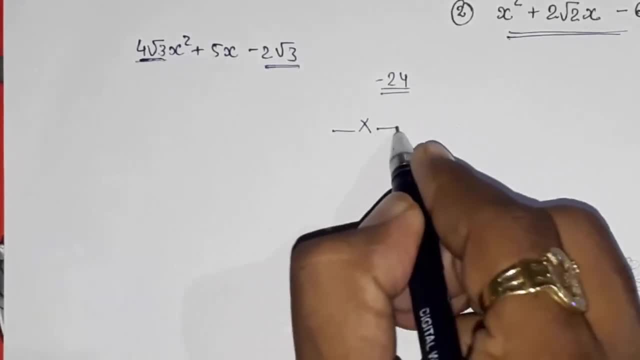 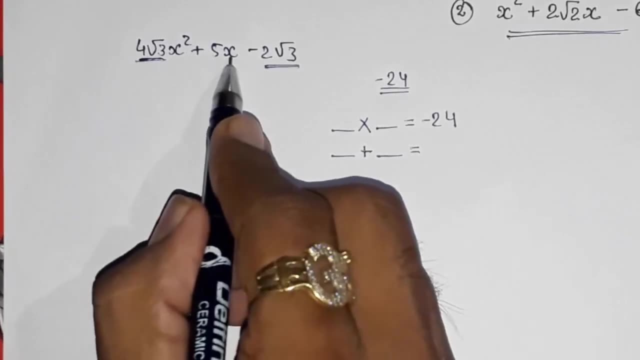 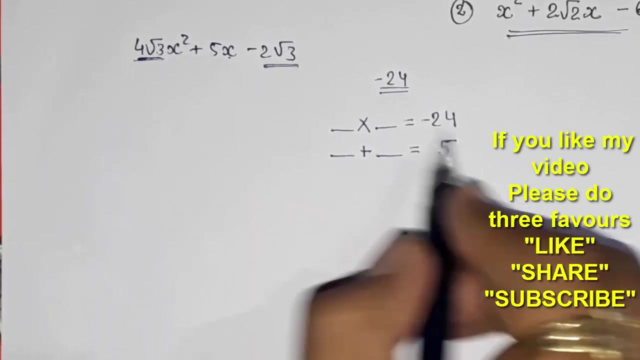 20.. 4 will be done. now we have to find out the factor whose multiplication will be minus 24, and addition will be the coefficient of- or you can say b, only b, a coefficient of x, that is plus 5. so what will be the factors? 8, 3 is at 24, and 8 minus 3, that will be 5. so 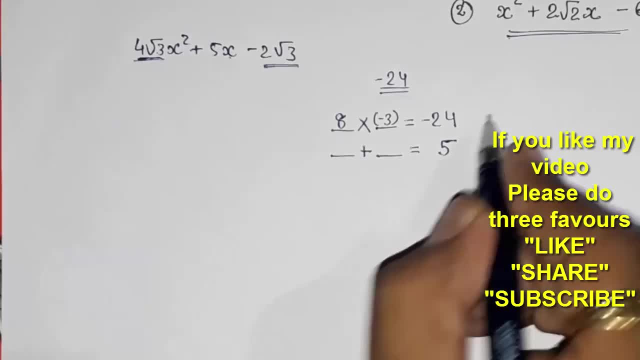 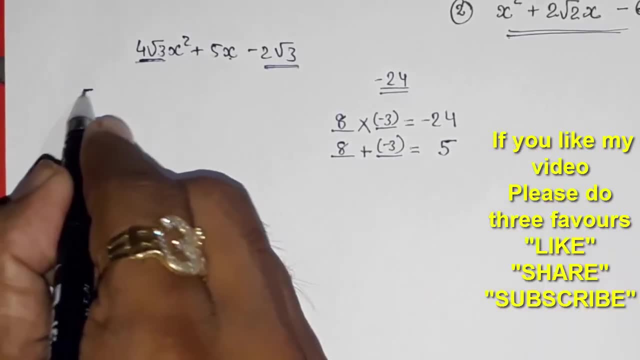 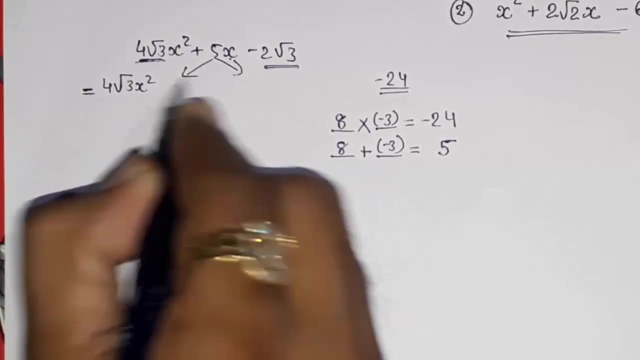 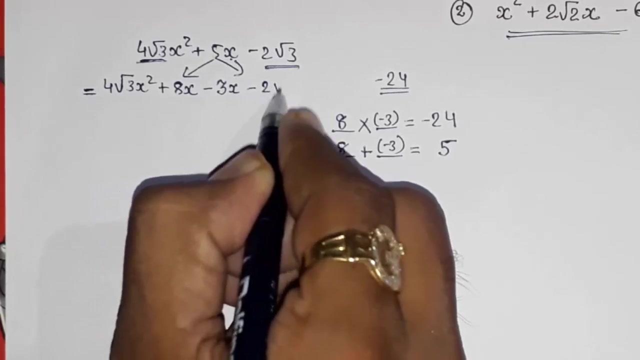 8 into minus 3, that will become minus 24. 8 plus minus 3, that will become positive or plus 5.. Now directly find out. keep the instead of 5, split the middle term as plus 8x, minus 3x and then again minus 2 root 3.. 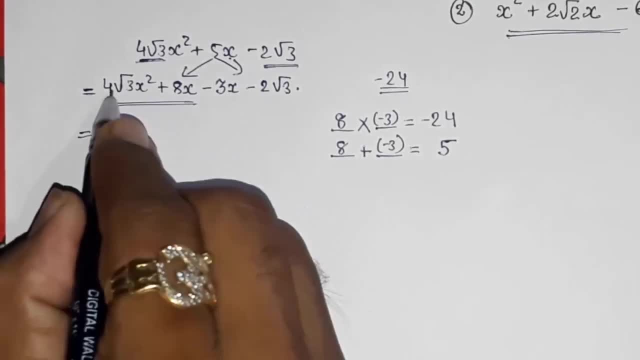 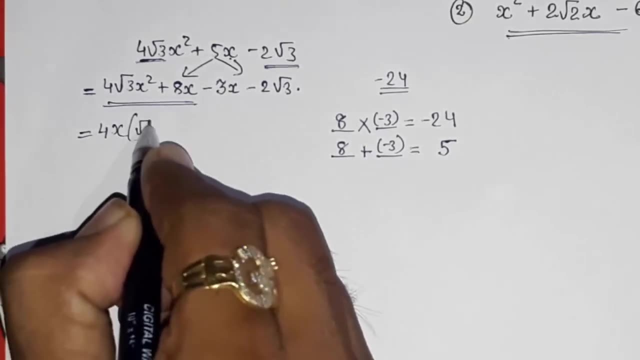 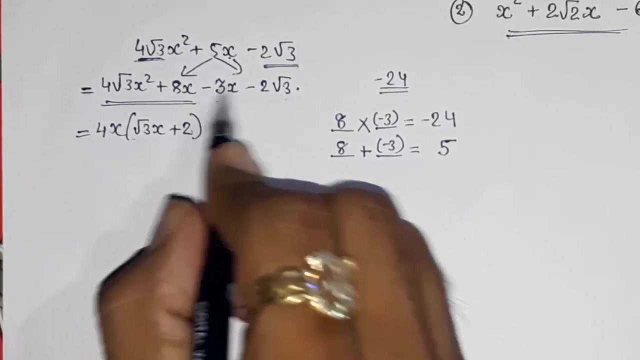 Now we have to find out the common from this 2 number. it's so simple: four and it's 4. two, pi g, forma 2, 2, 4, 44, 3x plus, and here will be 2. now take out common from these two numbers. minus is there. so first, 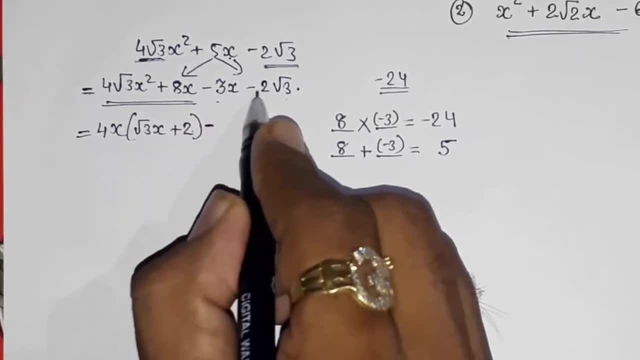 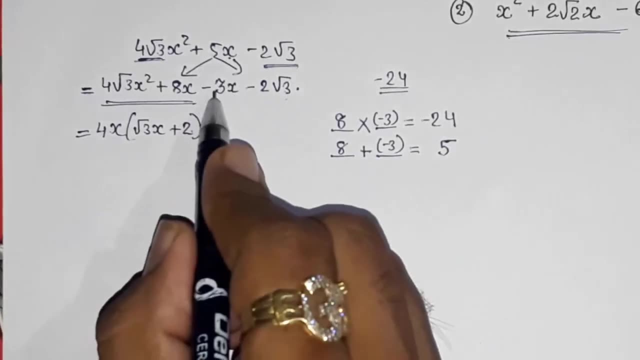 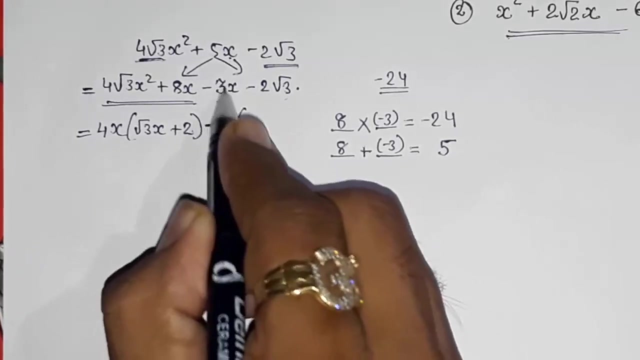 we will take out minus because we want to convert this plus. it was here, so here also we want plus. but here it's 3 and root 3, so the factors of 3 is actually root 3 into root 3, and here also 1 root 3 is there, so you can take out root 3 also common. now from this 1 root 3 is gone. so 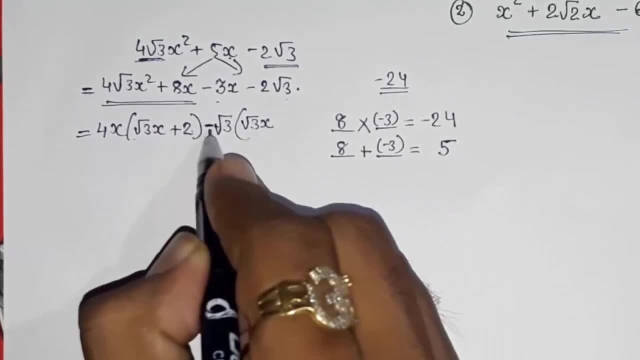 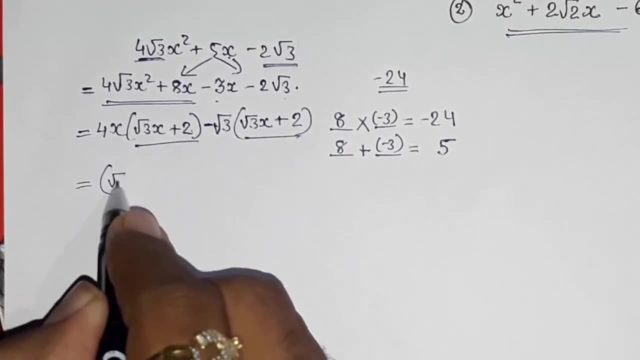 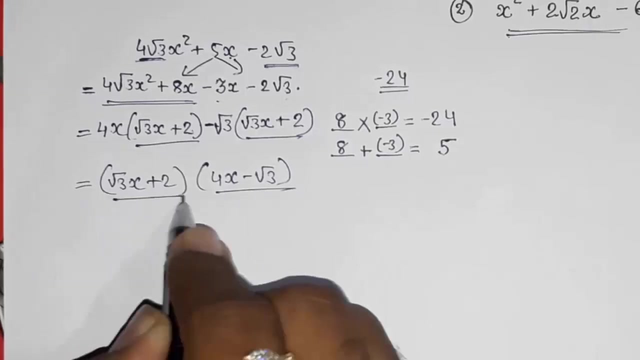 1 root 3 will be remaining and x and then this minus. we had taken out common, so plus 2. now you can see both the factors are same root 3x plus 2, and the other is 4x minus root. now these two are: 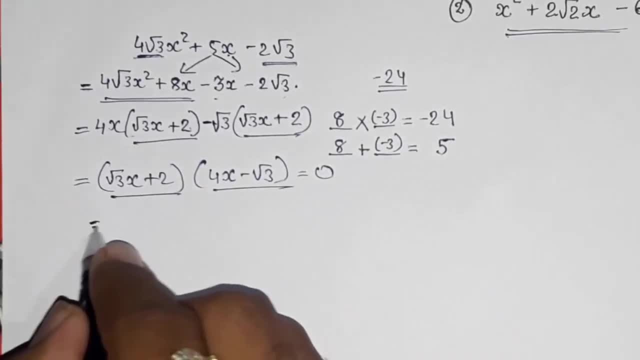 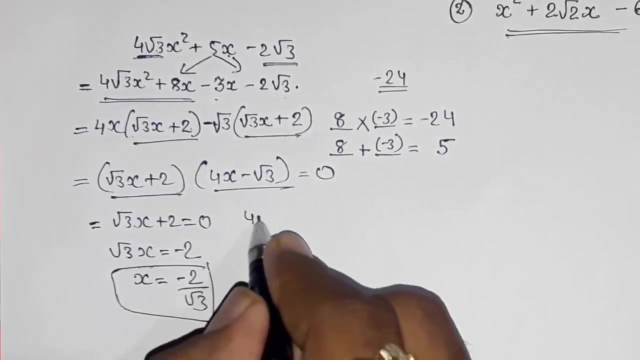 the factors. we want 0, so equal to 0. so here root 3x plus 2 is equal to 0. so root 3x is equal to minus 2. x is equal to minus 2 by root 3. this will be your first 0, and here this will be 4x minus root 3 is. 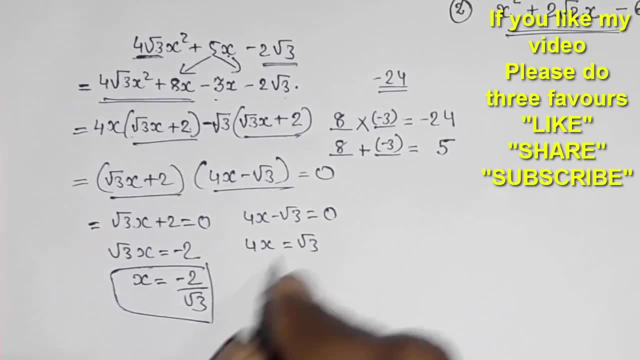 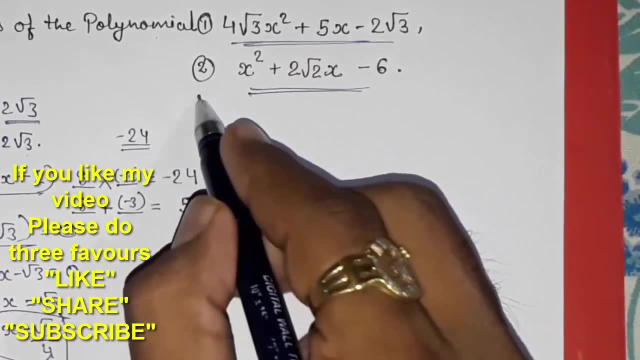 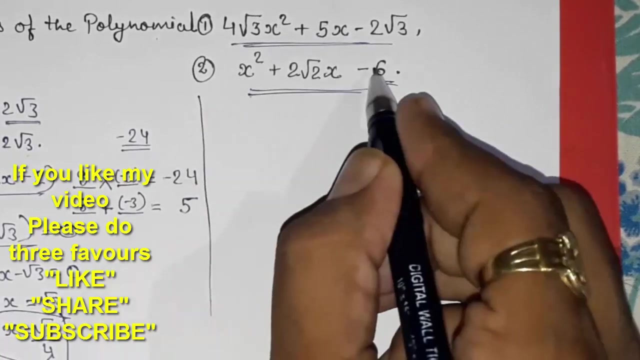 equal to 0, 4x is equal to root 3 and x is equal to root 3 by 4. so these are the two: 0 now for this. sum x square plus 2, root 2x minus 6. so here, 1 into minus 6 minus 6. so what we have to, we have. 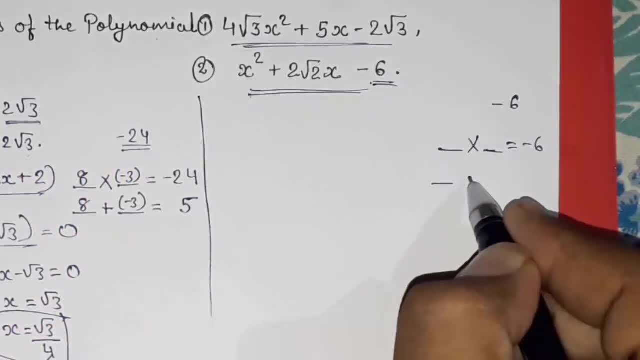 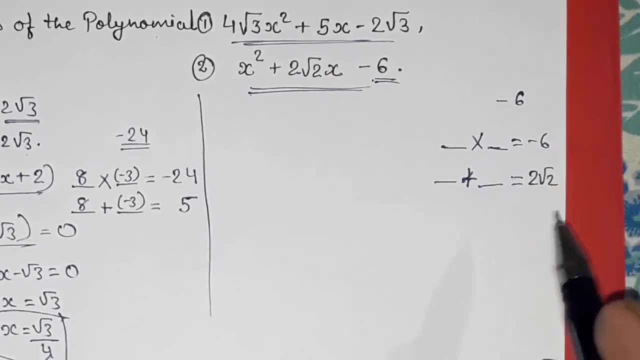 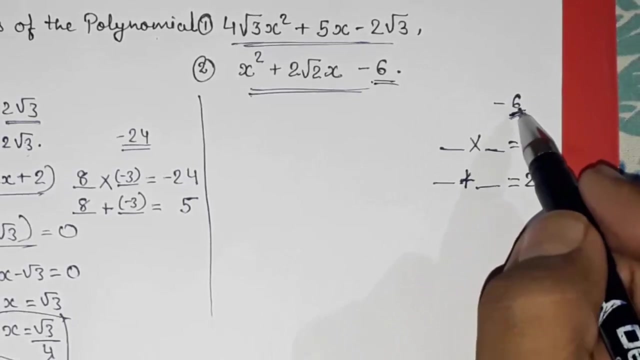 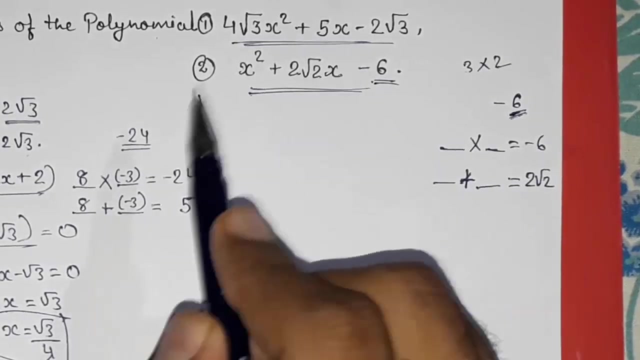 to find out the factors of minus 6, so that multiplication will be minus 6, but addition will be the middle number, that is, 2 root 2. now the problem arises. now we have to find out the factors of 6 first. we know factors of 6 will be 3 and 2, 3 multiply with 2. but we want 2 root 2. 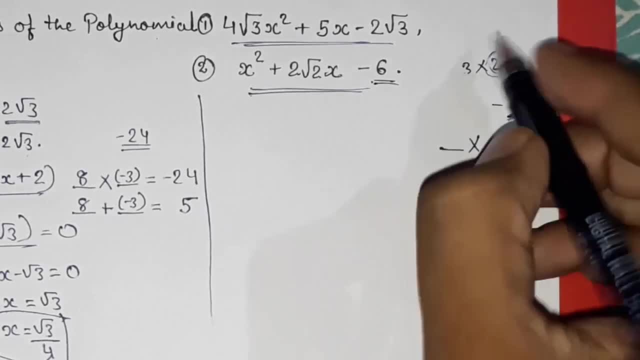 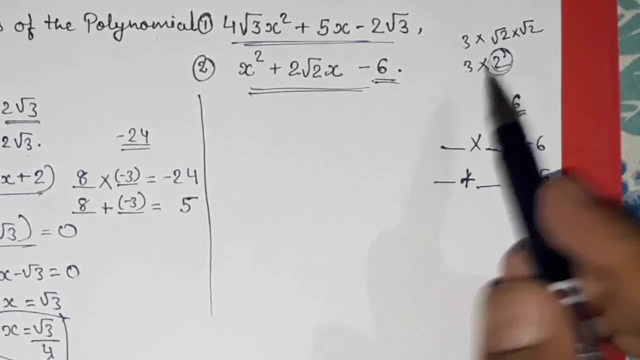 so root 2 is there. so again we have to find out the factors of root 2. that will be root 2, root 2 and this 3. now you can add or subtract out 3 into root 2 means you can make one pair of. 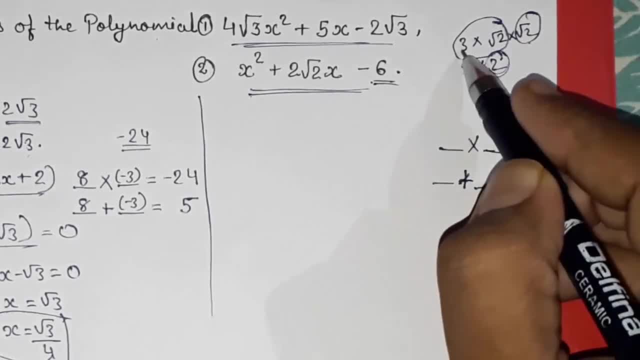 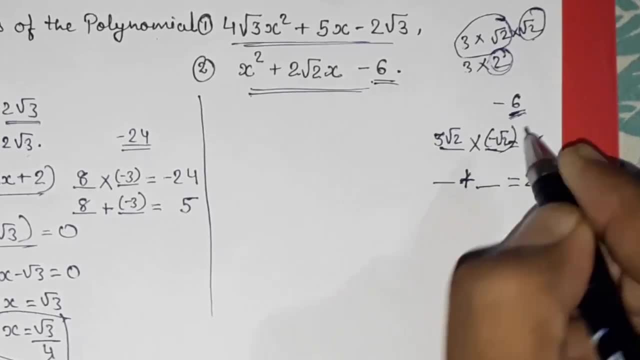 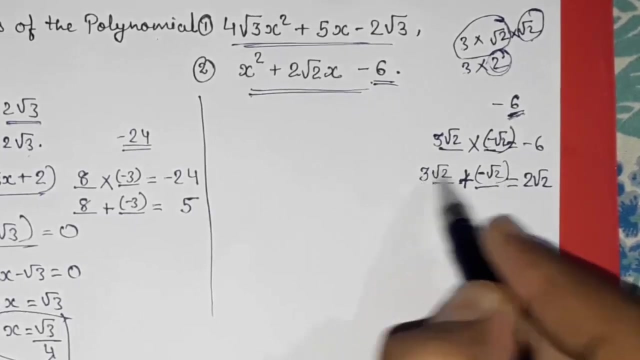 this and now: plus 3 into root 2 means 3 root 2 and minus root 2. yes, 3 into root 2. multiply with minus root 2. what will happen? minus 6 and 3 into root 2 plus minus root 2. subtraction 3 minus 1. 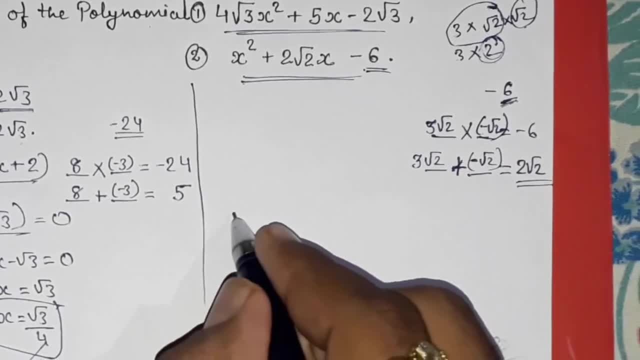 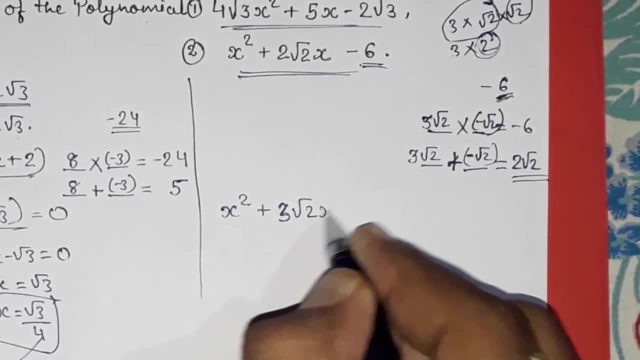 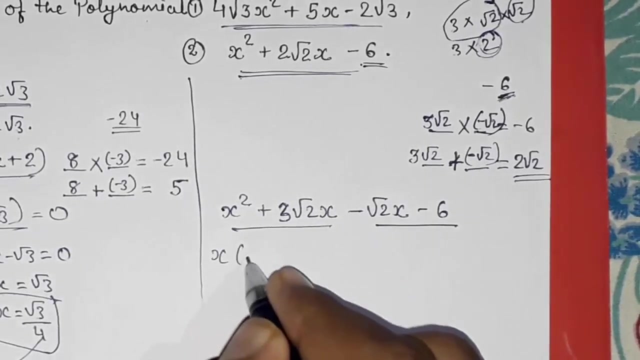 will become 2 root 2. yes, so we got the factors. i'm writing it here: x square plus 2, sorry. 3 root 2. x minus root. 2 x minus 6. now common. from this: 2 x common. x plus 3 root 2. now, first we want to take out minus common, because we here plus was there. so 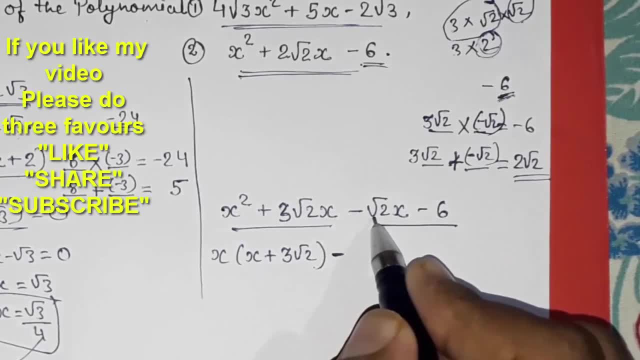 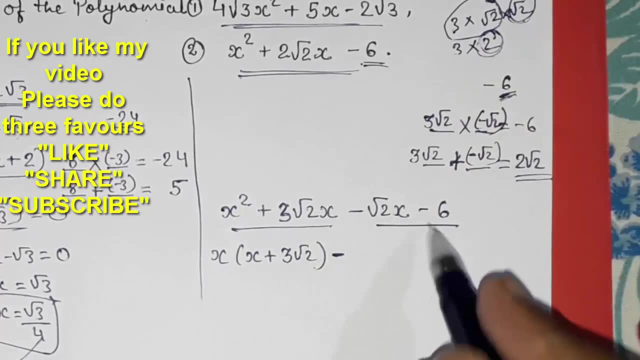 we have to change the sign now. we have to take out root 2. also look at the factors of 6. are 3 into root and so we can take out 1. root 2 common from this. so root 2 also common here. root 2 we had taken. 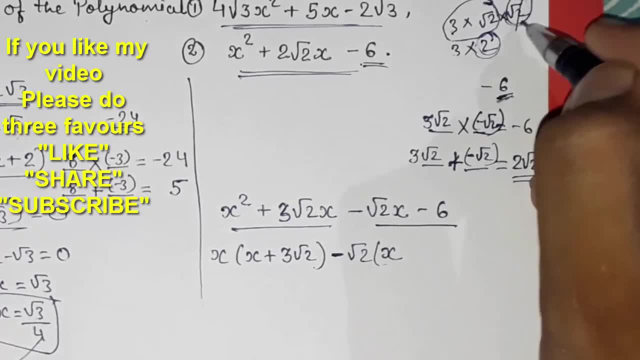 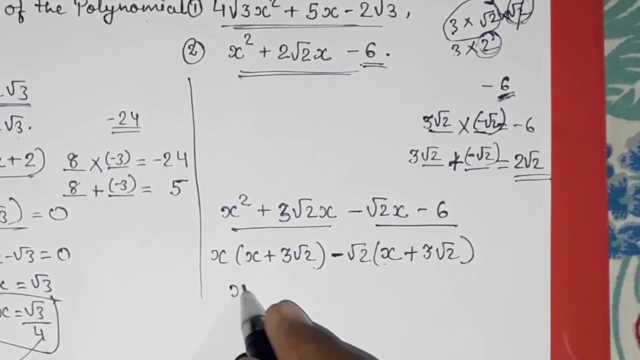 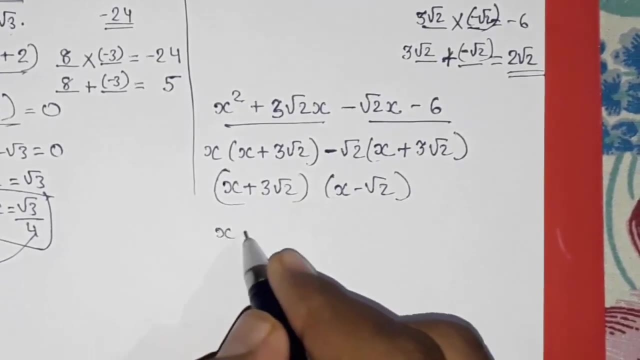 out common from x, and here out of this 6, only 1, this root 2 gone. so what will be the remaining number plus 3 root? now? what will be our factors? x plus 3 root 2 and x minus root 2. so x plus 3 root 2 is equal to 0. so X will be equal to 0.